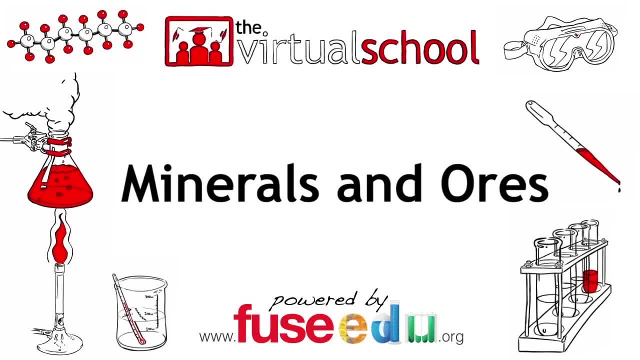 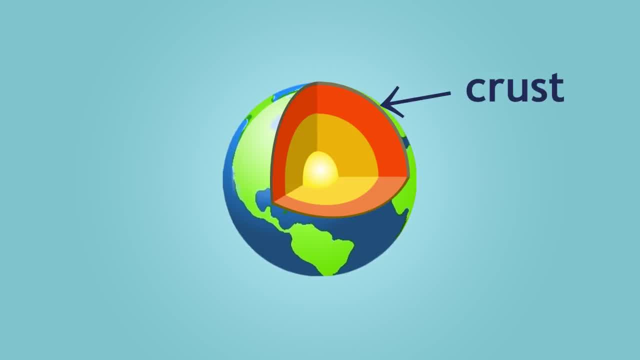 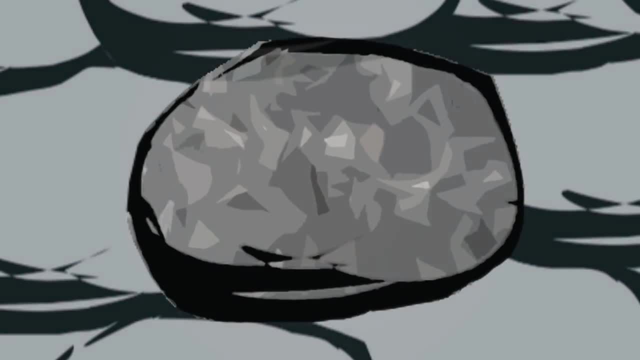 In this lesson, we will learn about minerals, ores and how minerals can be extracted from ores. As you may already know, the earth's crust is made of rocks. If you look closely at a rock, you will see that there are many different bits. Some bits are dull, whereas 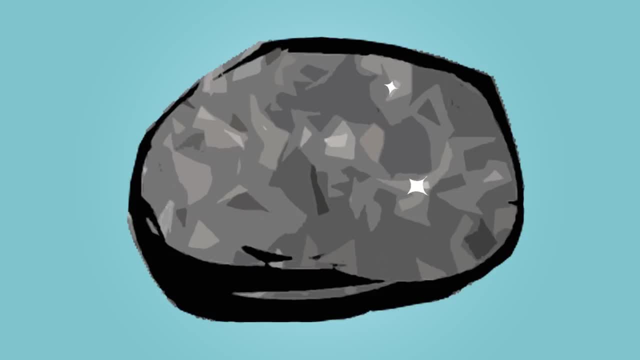 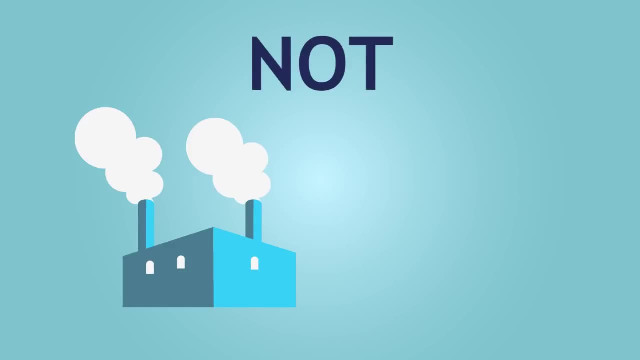 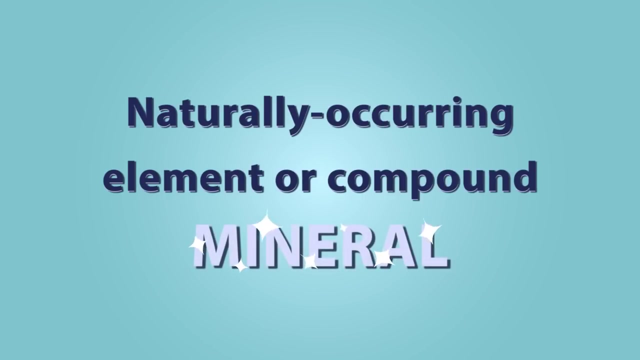 other bits are rather shiny. The main idea here is that all these components occur naturally, In other words, they are not made in a factory or by a human being. A naturally occurring element or compound is known as a mineral. Ore is simply a rock containing a high percentage. 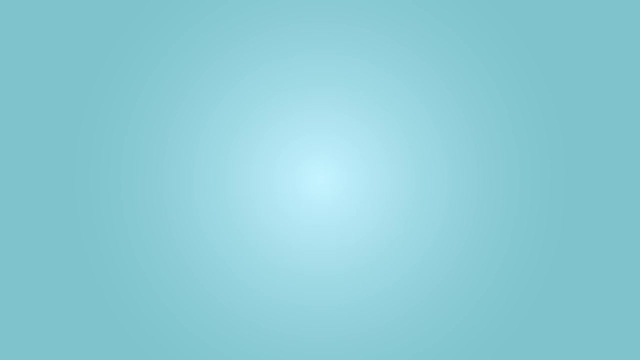 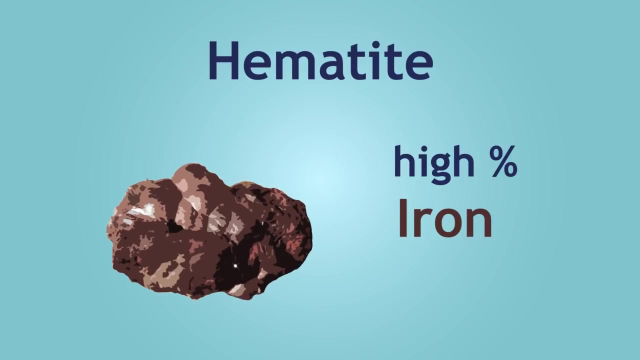 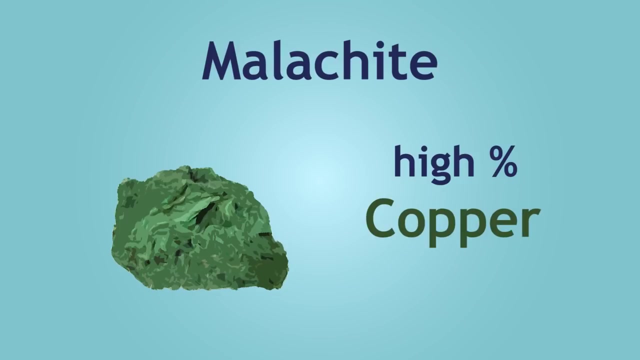 of a certain mineral. For example, hematite contains a high percentage of iron. The extraction of iron from hematite is done in a blast furnace. Malachite contains a high percentage of copper. Cinnabar contains a high percentage of mercury. 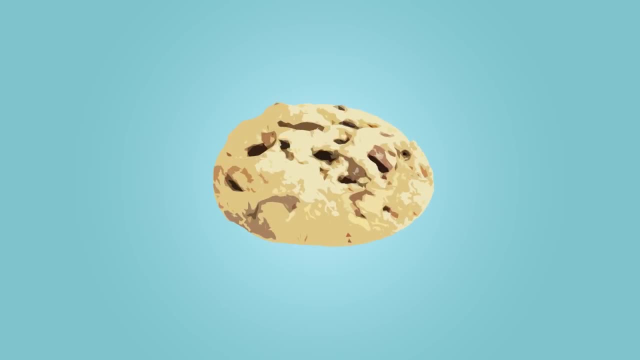 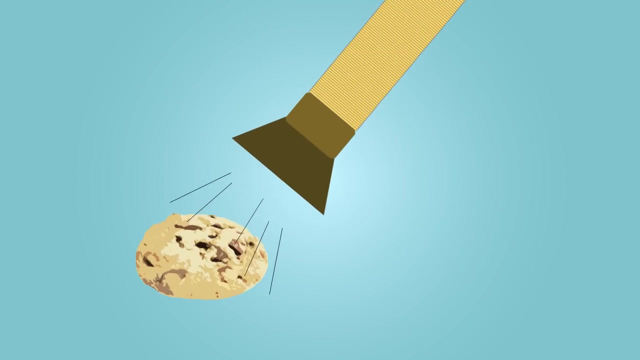 We can think about an ore a bit like a chocolate chip cookie. We really want the chocolate. If there are more chocolate chips in the cookie, then the extraction process would be more economically beneficial, as more minerals, in this case, the chocolate, can be obtained. 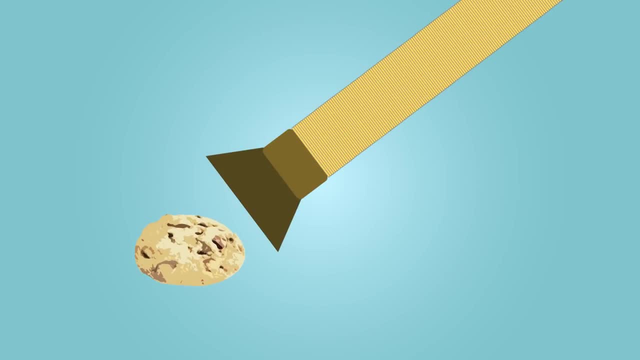 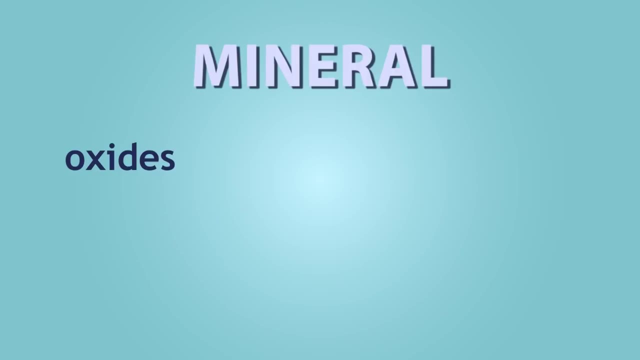 If there are fewer chocolate chips, then the extraction process may not be as economically beneficial. For the most part, the minerals are oxides, carbonates or sulphides of the metal of interest. Some ores of nonmetals include quartz, which contain a high percentage of silicon in the 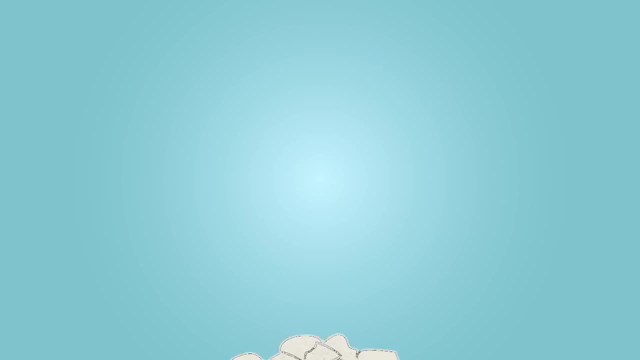 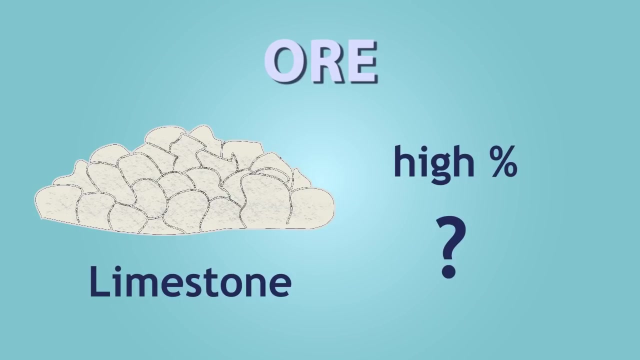 form of silicon dioxide. Limestone is also an ore. Can you remember what is found in a high percentage in the chocolate chip percentage in limestone? Pause, think and continue when ready. The answer is calcium carbonate. Limestone contains a high percentage of calcium, but 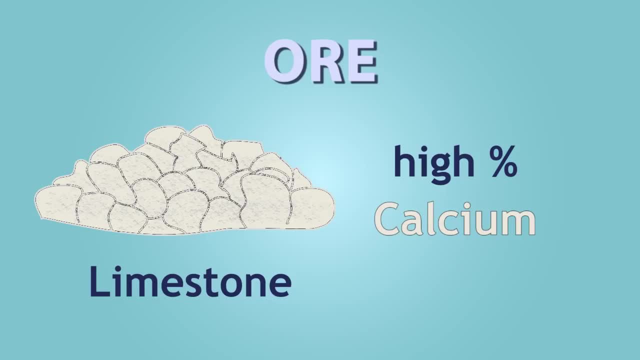 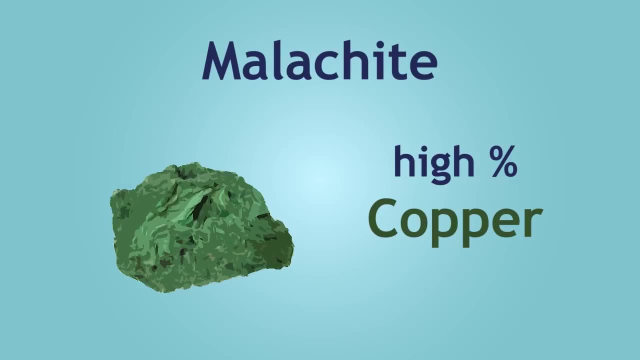 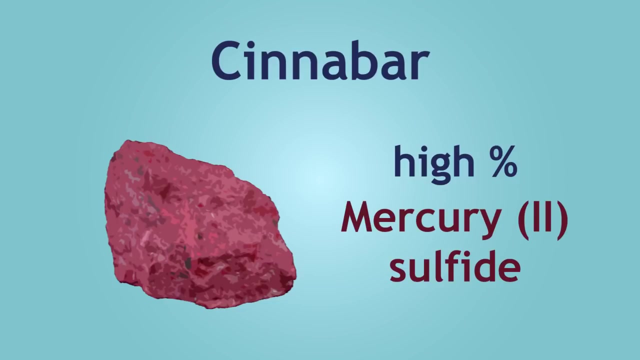 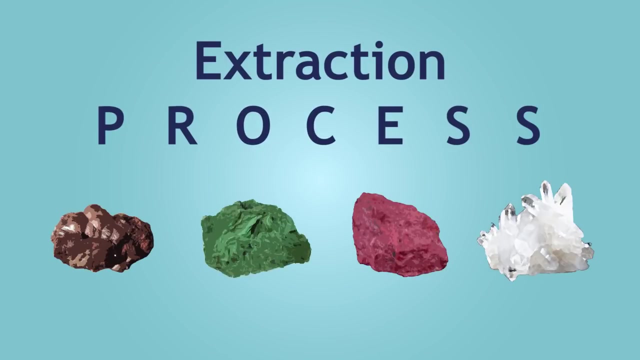 calcium exists as calcium carbonate. The iron in hematite is mostly iron oxide. The copper in malachite is mostly copper carbonate. The mercury in cinnabar is primarily found as mercury sulfide. The extraction process for each ore can vary, but the key idea here is that the 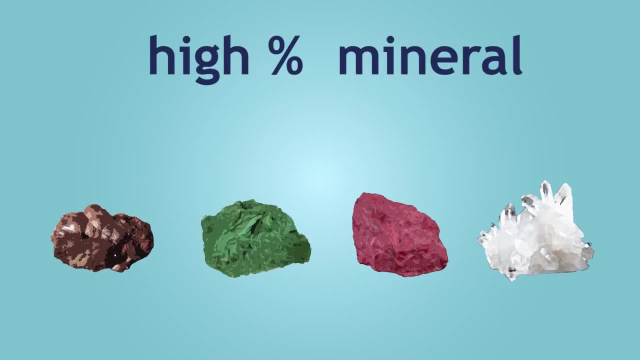 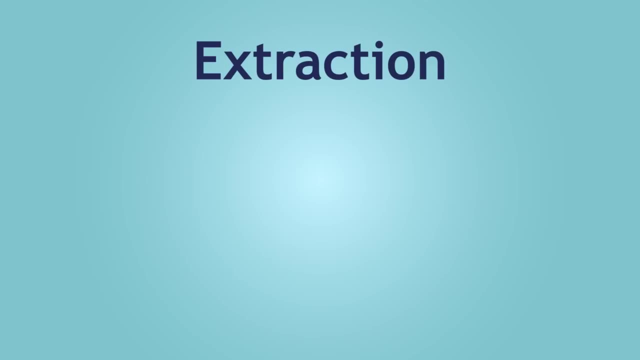 mineral must be present in a high enough percentage, or else the process would not be very economically beneficial. Now, before we can extract a selected metal, we must first consider the reactivity. by looking at this reactivity table, The most reactive metals are at the top of. 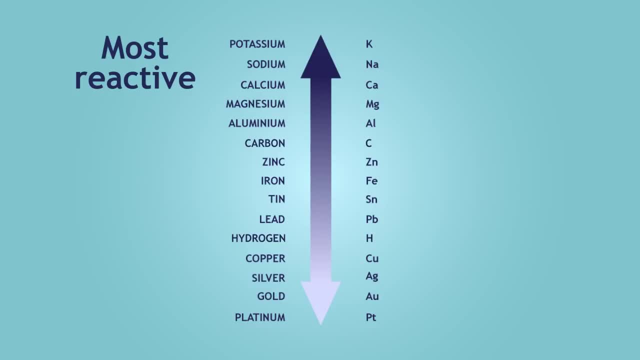 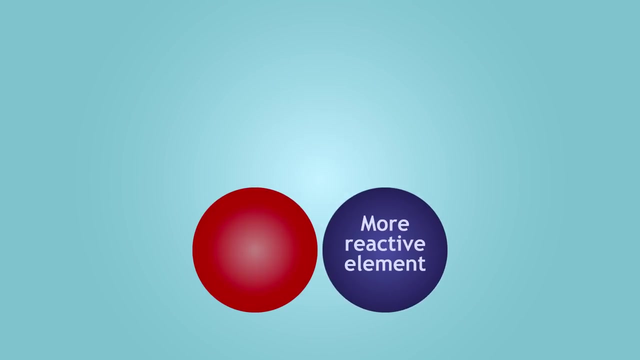 the series and the least reactive at the bottom of the series. Although carbon and hydrogen are not metals, they are still included in the table for comparison purposes. A more reactive element can displace a less reactive element in a compound. Can you remember what? 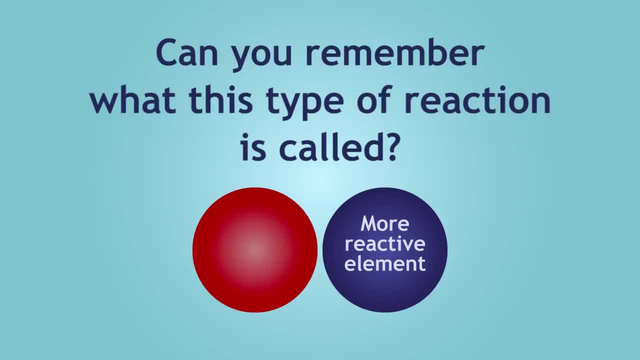 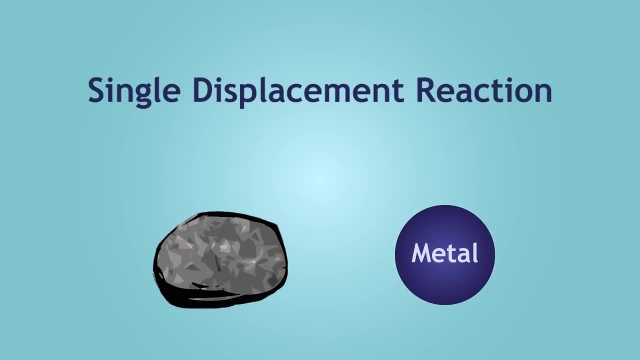 this type of reaction is called Pause, think and continue when ready. The answer is a single displacement reaction. So to extract a metal from an ore, a single displacement reaction must occur. We can mimic the extraction of copper from malachite using 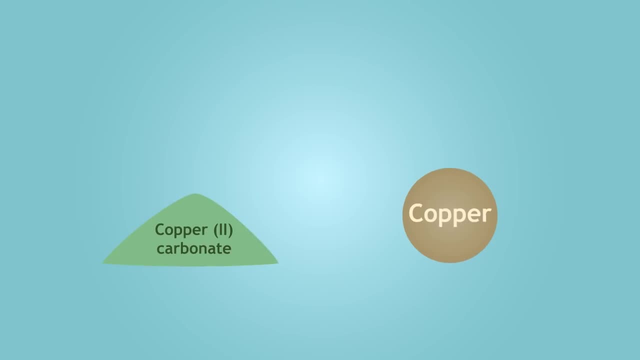 copper two carbonate powder. Copper two carbonate is a green solid that thermally decomposes to fluorine. It forms copper two oxide and carbon dioxide upon heating. Copper two oxide is a black powder and, believe it or not, we can actually extract copper metal from copper two oxide. 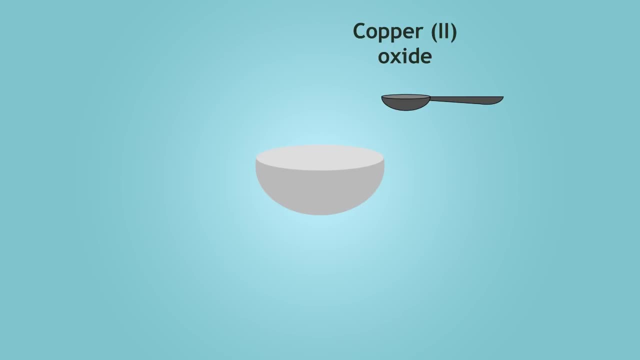 Place three spoonfuls of copper, two oxide, in a crucible and one spoonful of charcoal, which is essentially carbon. Heat this using a Bunsen burner with the crucible lid slightly ajar for approximately five minutes. While that is in progress, why don't you grab a?